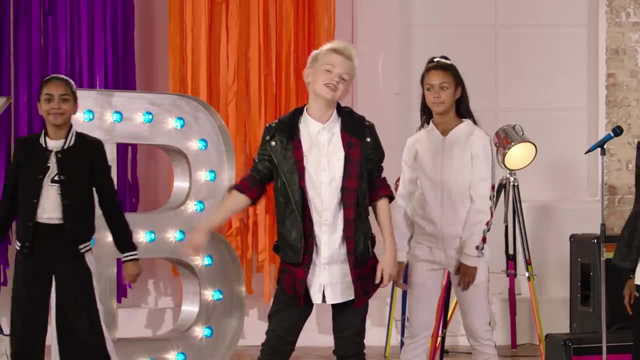 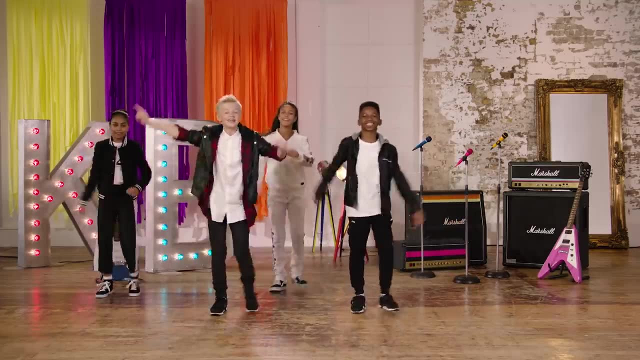 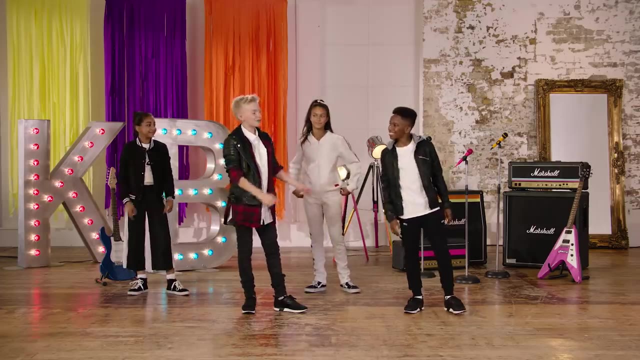 Has everybody got that? Then let's go from the top Five six. All you have to do is stay a minute, Just take your time. The clock is ticking, so stay Now. I'm going to pass you over to Ashton, who will be doing the second half of the chorus. 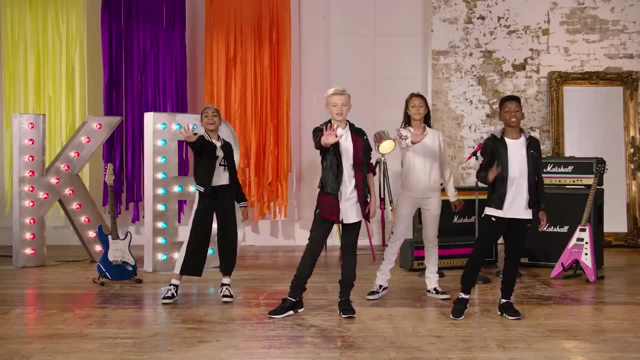 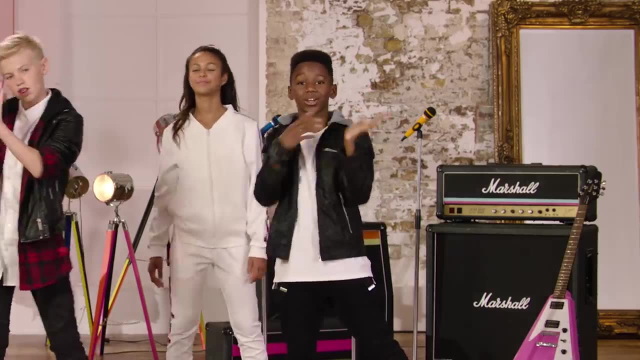 Thanks, Max. So you've just gone, stay. After that you're going to crouch down like you're doing a stretch, but with your hands flexed. Flex means to have a 90 degree angle With your hand. So that means you've gone stay. All you've got to do is 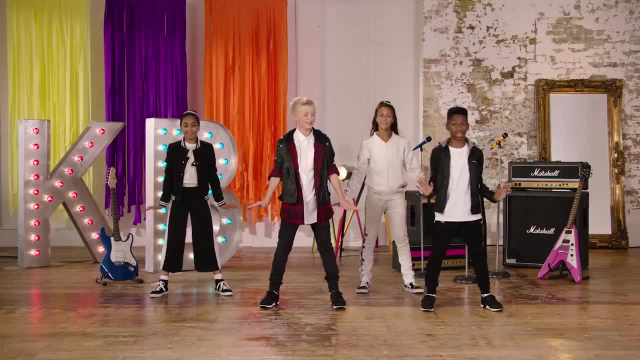 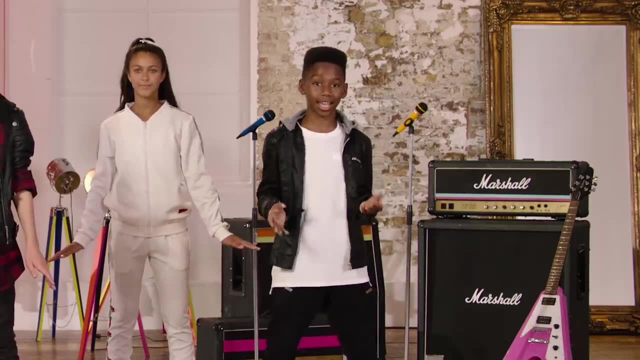 After that, you're going to pop up on the word wait with your hands still flexed. I feel like a penguin, Ashton. After that, you're going to break the word second into two parts. Second, On the first bit you're going to hop and your hand across your body. 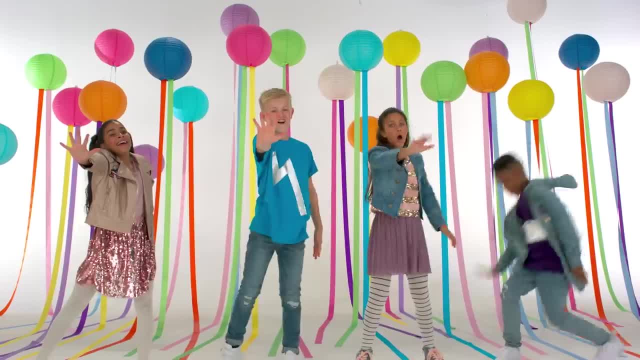 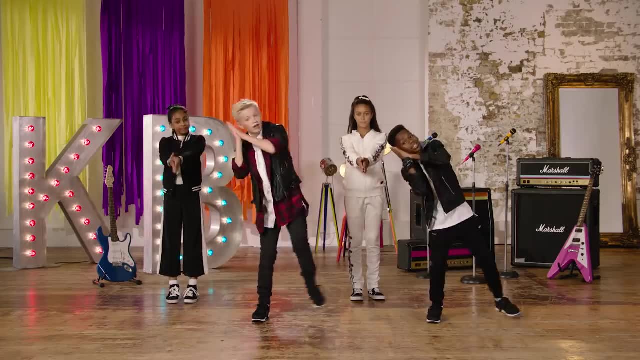 The second bit: you're going to bring your hand across and your foot down. Second After that, like the word say, you're going to bring your hands together and bring it to the side of your face and stretch your leg out. Then you do the same move on the other side. 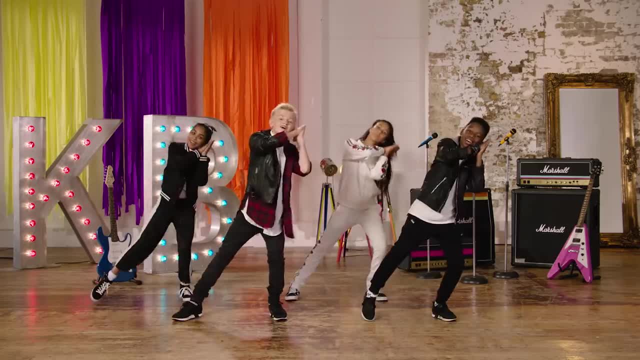 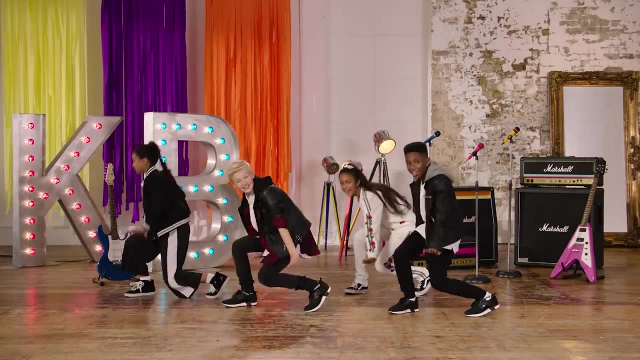 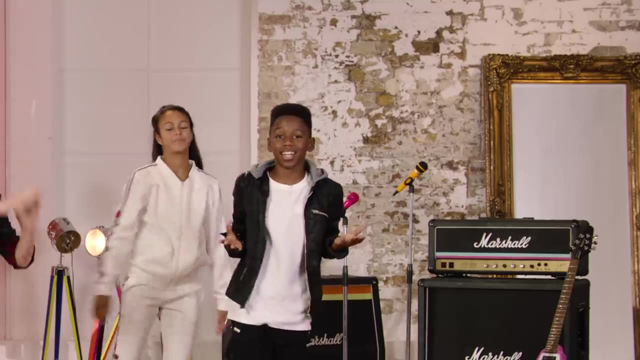 That would be on the words your hands on man. Your hands on man From the top, Slowly, Five, six. All you got to do is wait a second. Your hands on man. Then, like before, you're going to go to the clock. 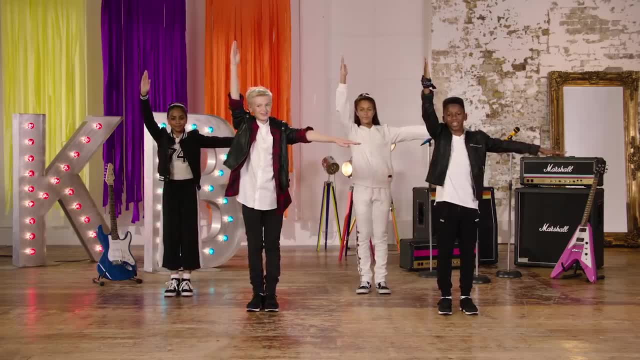 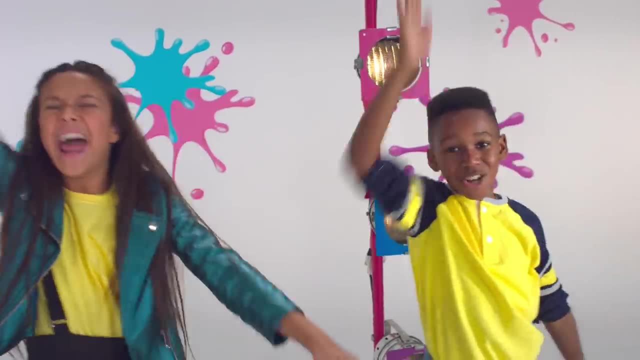 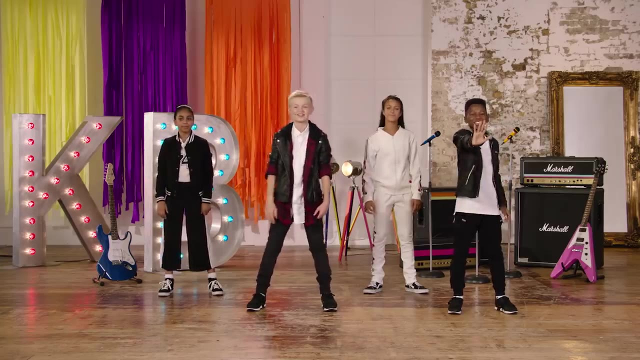 Like this, And then on the words ticking, you're going to go down Ticking, Then back to the original move of stay, But then in the music you're going to hear this sound that sounds like So you're going to bring your hand back to your body. 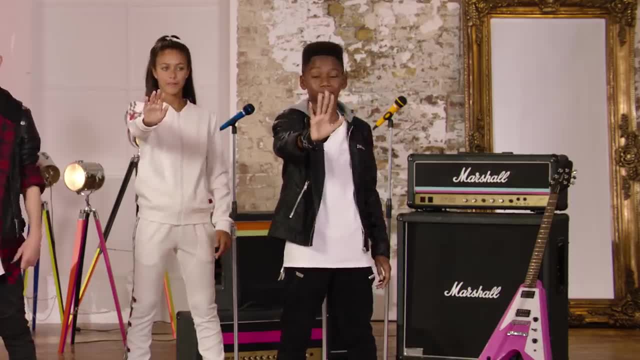 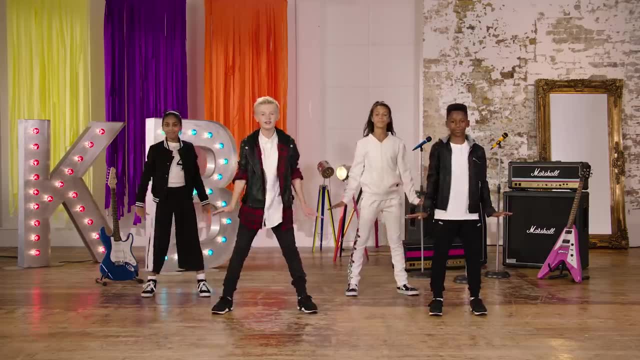 But every time you come back you're going to pretend you're hitting a ball on each beat. At the end you're going to go heel toe with your feet and then pull away And then back. So all together that is pop, pop, pop, pop, heel toe back.